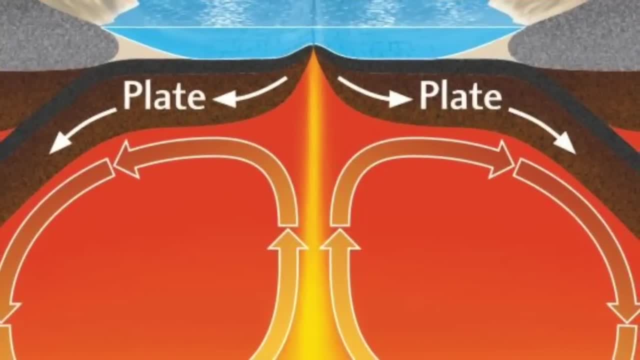 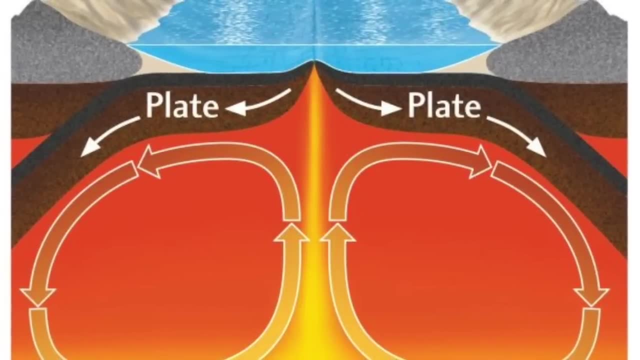 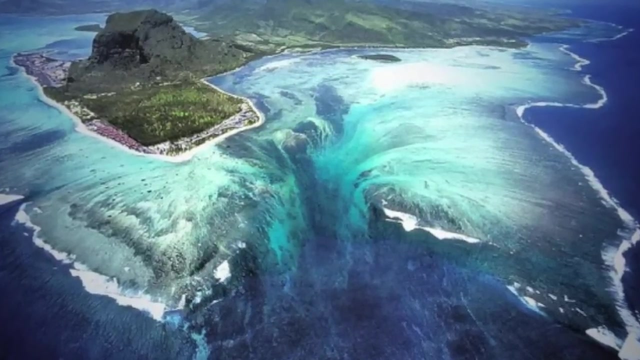 Geological oceanography is a broad field and has many subdivisions, including geophysics and plate tectonic studies. Geological oceanographers study the basic structure of the ocean floor, as well as more specific features such as rises and ridges, sea mounts, abyssal hills, the oceanic crust, sedimentation, erosional processes and volcanism. 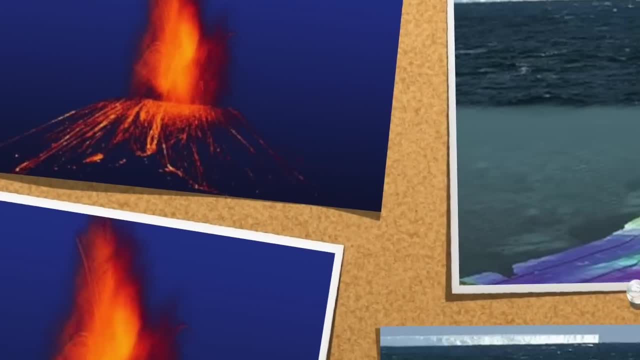 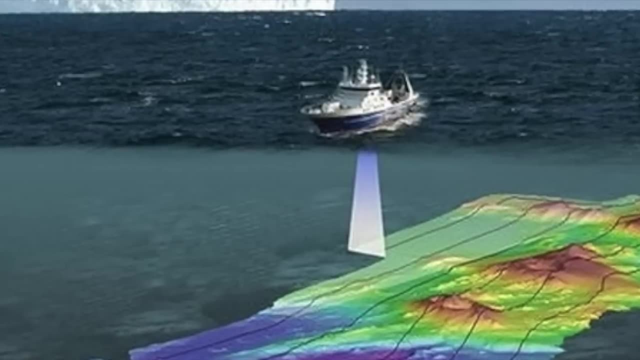 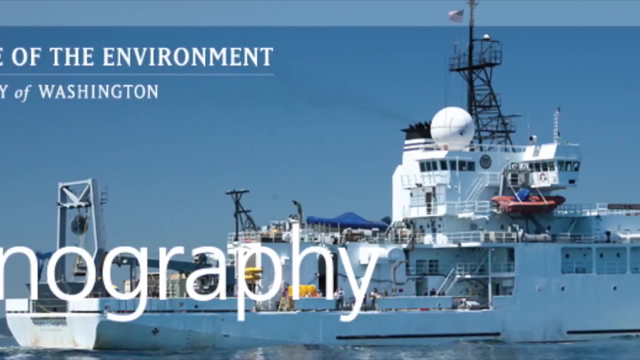 Unlike other fields of oceanography, geological oceanographers do lots of research as opposed to applied sciences. Their main job is mapping the sea floor and studying the structures of the ocean floor. Contrary to what one might think, there is not an abundance of colleges in the United States that offer oceanography. 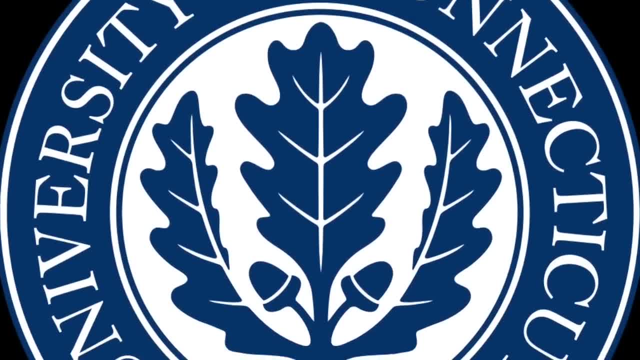 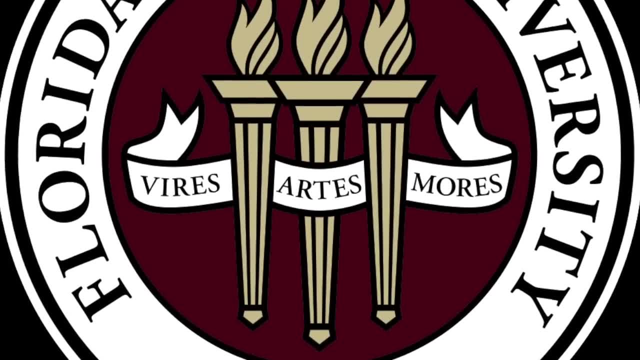 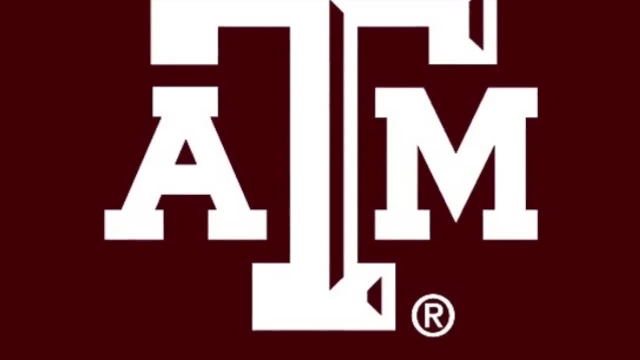 specifically geological oceanography. Throughout the country, mainly located on the coasts, are about 30 different colleges and universities that offer geological oceanography. These include the University of Washington, University of Connecticut, Florida State University, Texas A&M University, Oregon State University. 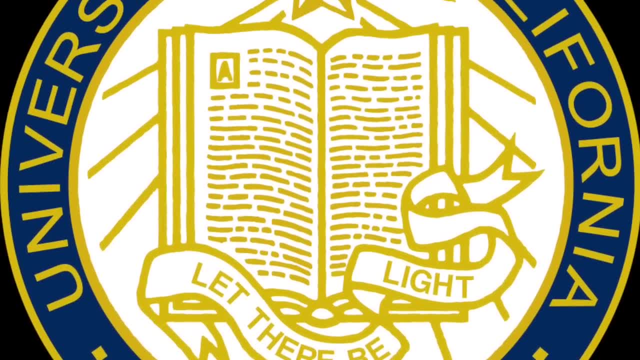 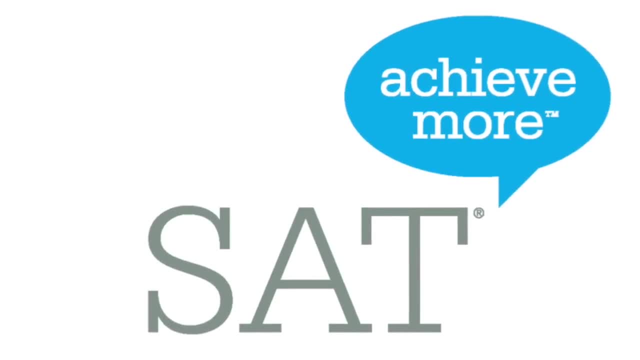 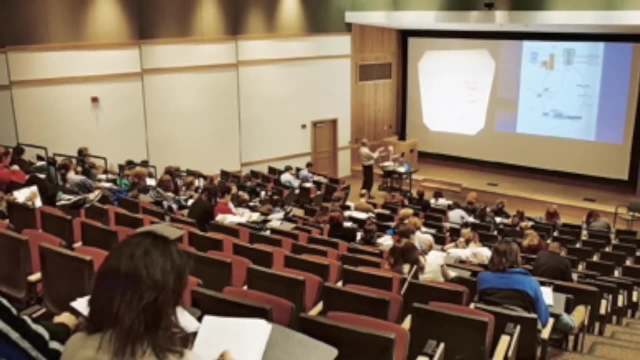 and several University of California schools. Although colleges require a multitude of test scores and grades for acceptance, most do not have any specific requirements for being a part of geological oceanography. However, it all depends on the school. Some schools may have a program that accepts any already enrolled college student. 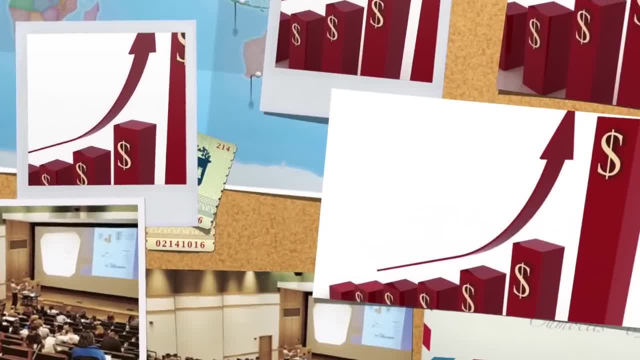 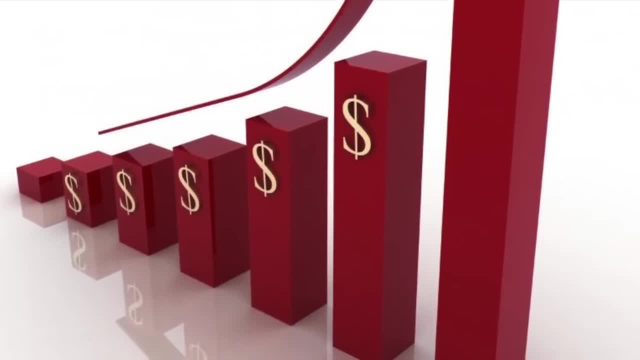 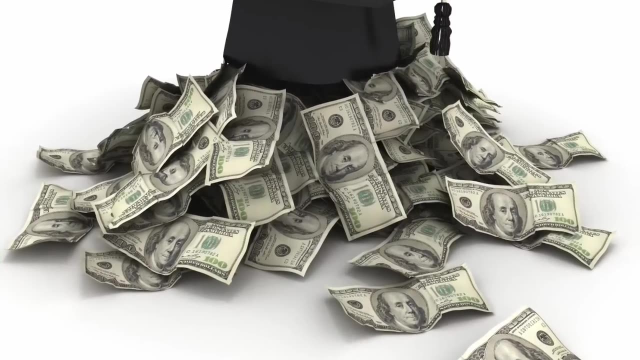 while others may require specific grades to be accepted into the oceanography program. Also depending on the school and program, is cost. College prices for geological oceanography can range from $10,000 to $50,000 per year. A college in California might cost more than a college in Florida, for example. 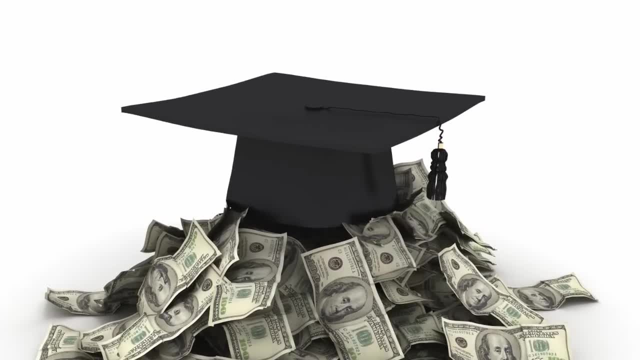 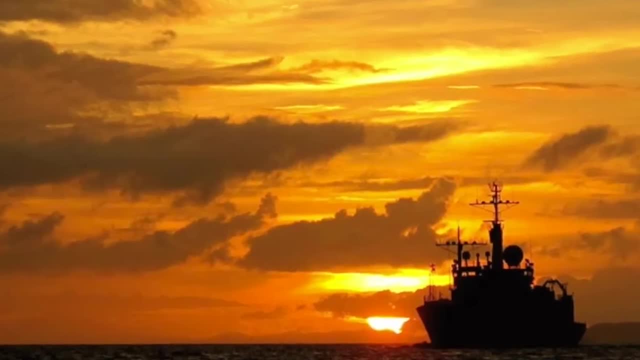 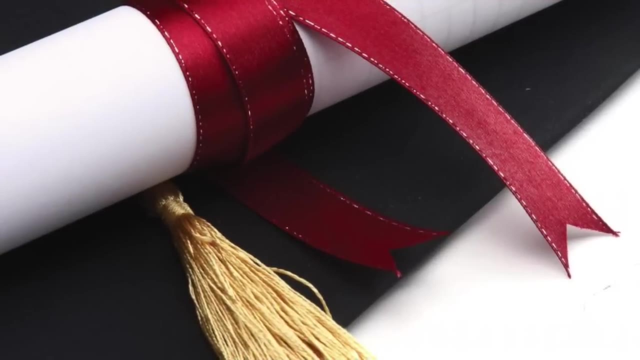 This variance in price, however, does not represent the quality of education. The Florida school may have a program just as good or even better than the California school. Unlike some specialized subjects having to do with the ocean- geological, oceanography, jobs- do not require too much specific educational milestones. 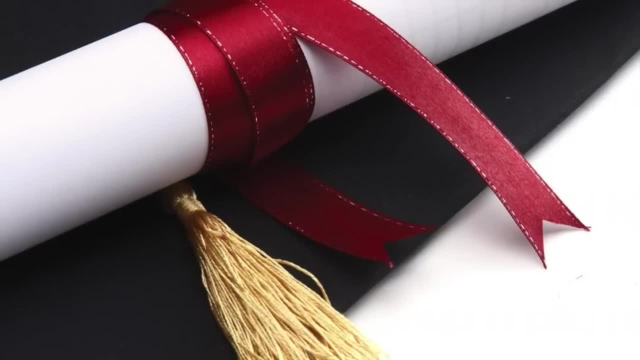 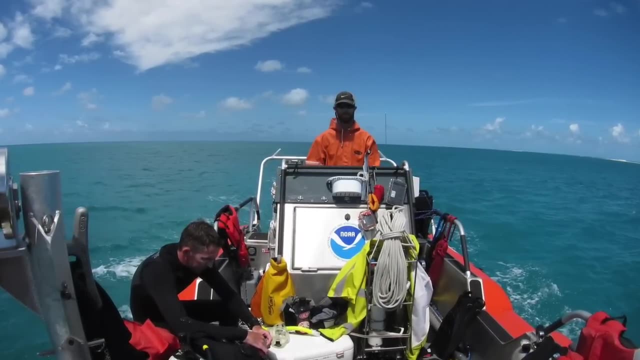 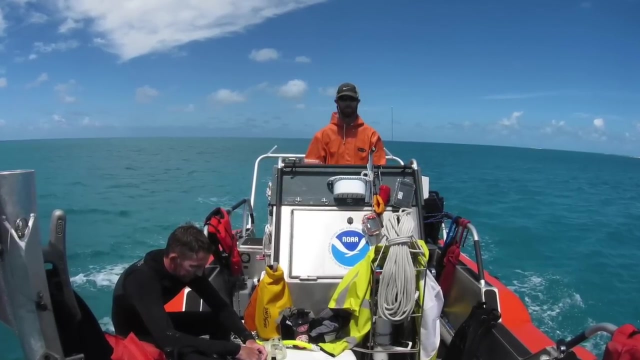 For most jobs, a general oceanography degree is required. However, specifying in geological oceanography or having a master's or doctorate degree will give you an edge in the workforce. There are around 250 programs and institutes in the US that study the ocean using geological oceanography. 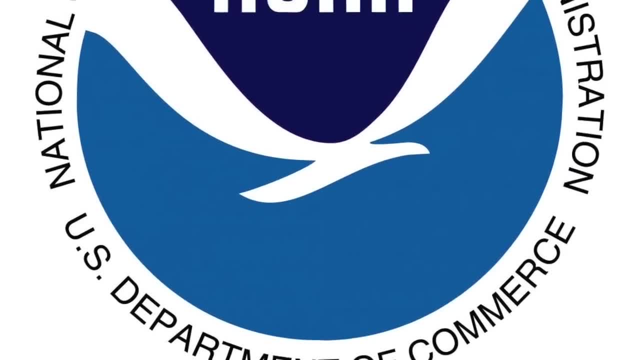 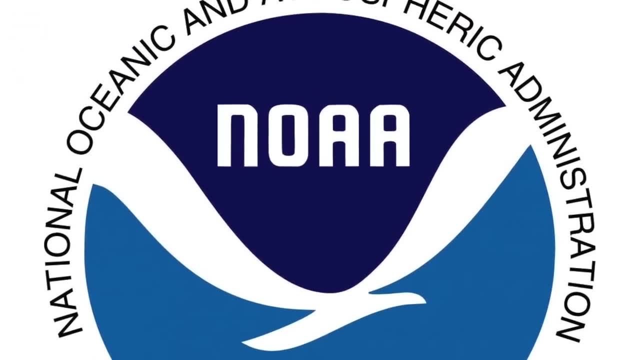 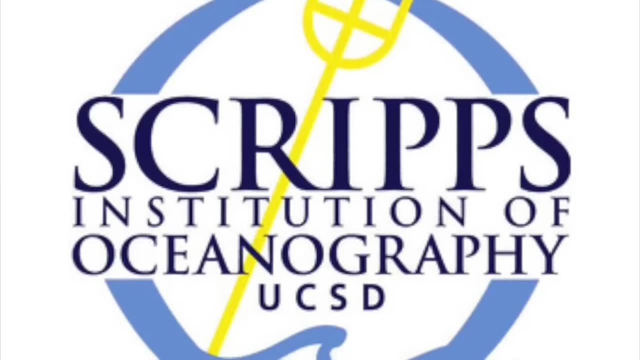 many of which offer both paid and non-paid internships and fellowships. The majority of these take place in the summer or spring. The National Oceanic and Atmospheric Administration, Ocean Exploration Trust, Harbor Branch Oceanic Institute. Scripps Institute of Oceanography. 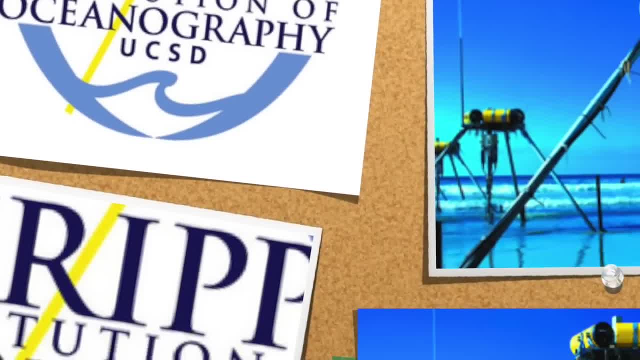 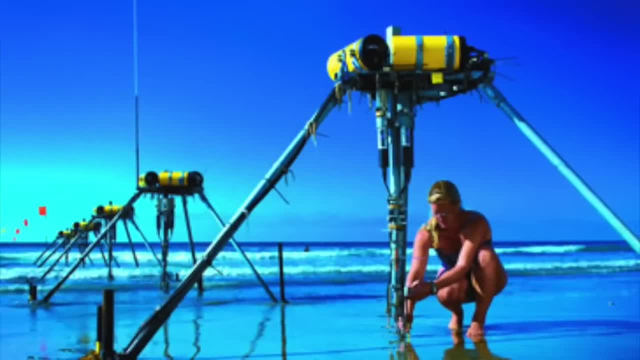 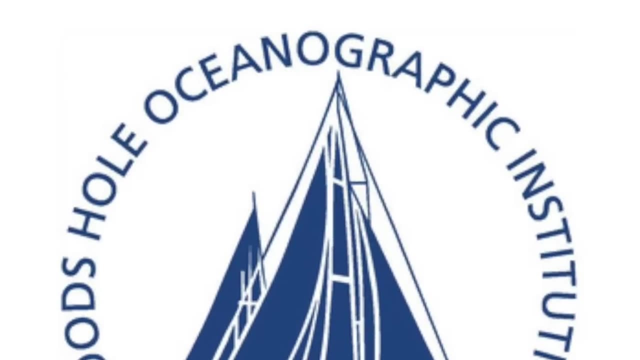 and Woods Hole Oceanographic Institute are just a few of the institutes that offer internships to both college students and graduates Out of the 250 institutions, many of which are also offering more permanent employment for geological oceanographers. Scripps Institute of Oceanography in San Diego, California. 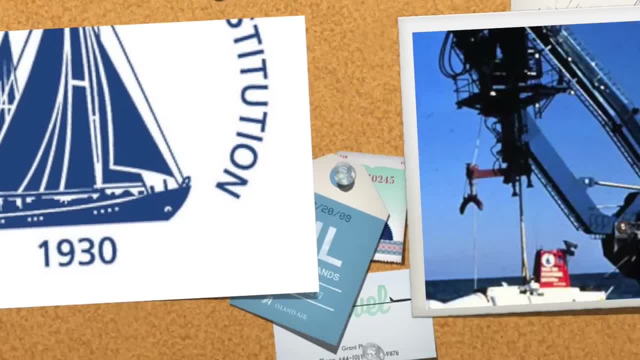 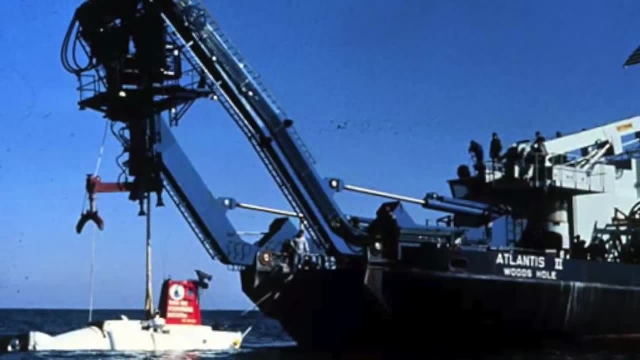 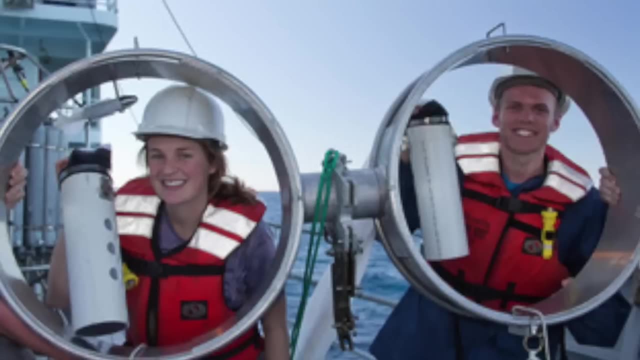 and Woods Hole Oceanographic Institute in Woods Hole, Massachusetts, are two of the largest and most notable institutes that are almost always hiring New employees and researchers. Colleges such as University of Miami, University of Washington and Oregon State University are also hiring for research positions. 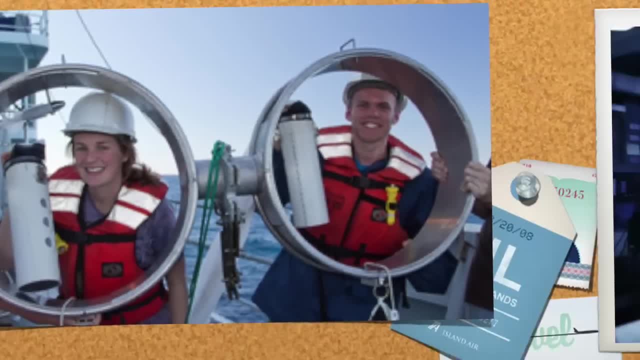 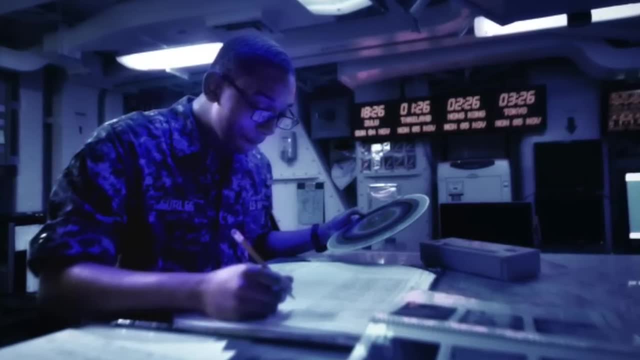 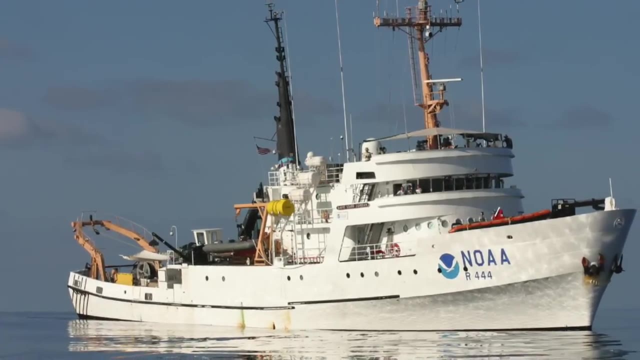 Geological oceanographers can also be in demand for jobs with the United States Navy. They can be helpful for planning routes of ships, especially submarines. The average annual salary for a geological oceanographer with a bachelor's degree ranges from $33,000 to $49,000, depending on level of expertise and the specific job. 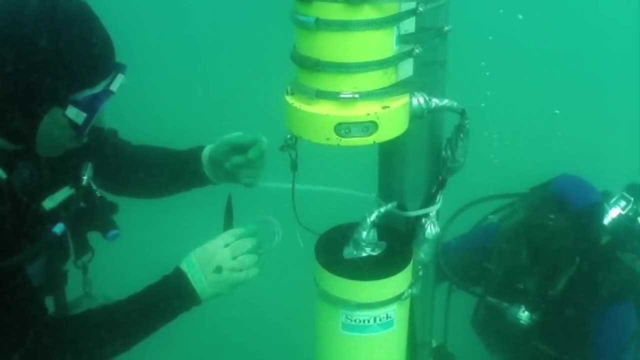 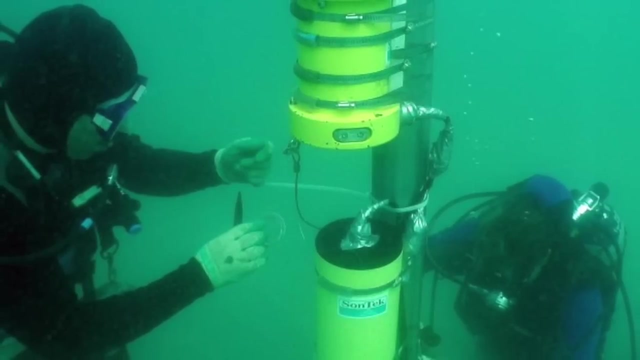 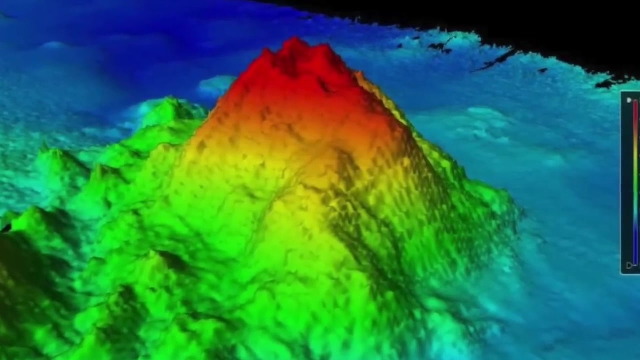 Applicants with a master's or doctoral degree may be offered a higher yearly salary. Although geological oceanography has a wide range of topics to study, the basic idea of finding out more about the ocean's floor is fascinating. Surprisingly, there is not too much to do in order to become a working geological oceanographer. 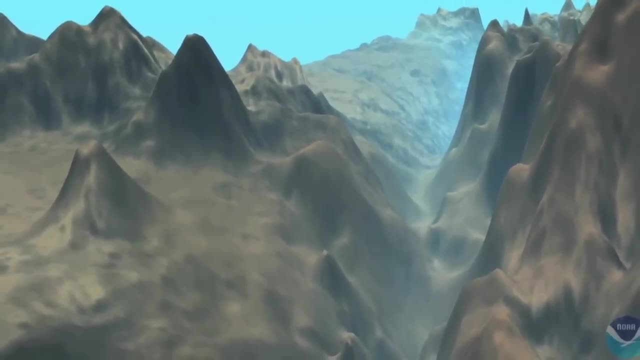 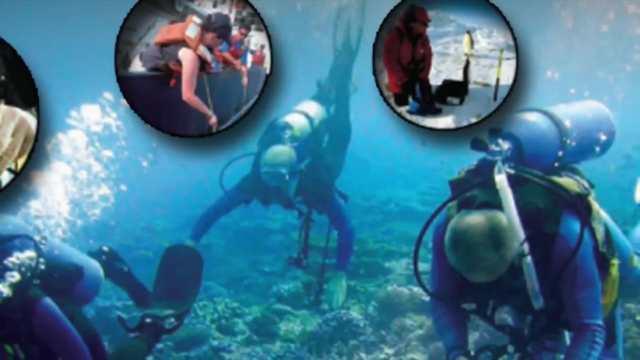 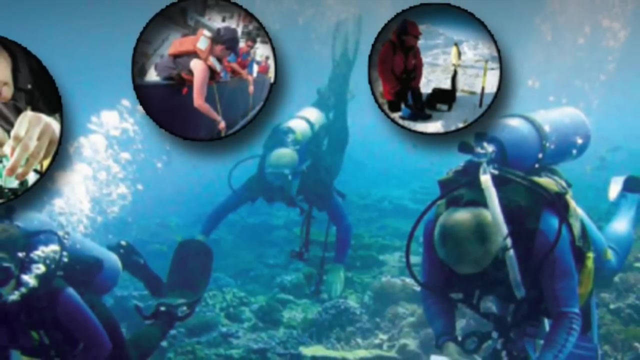 With the wide range of college programs, becoming a geological oceanographer is not too far out of grasp. Learning about the different possibilities in this field only made me more interested in studying this specific subject in college. I would love to learn more about how the ocean works from the bottom up.